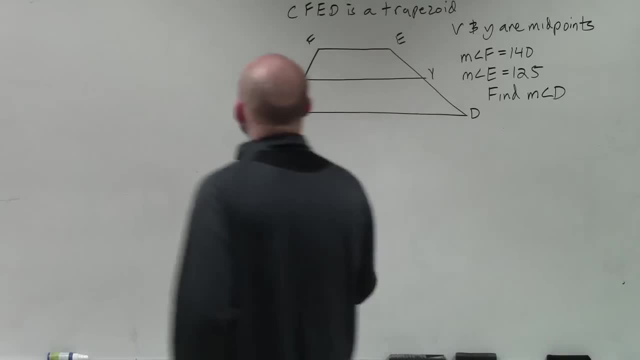 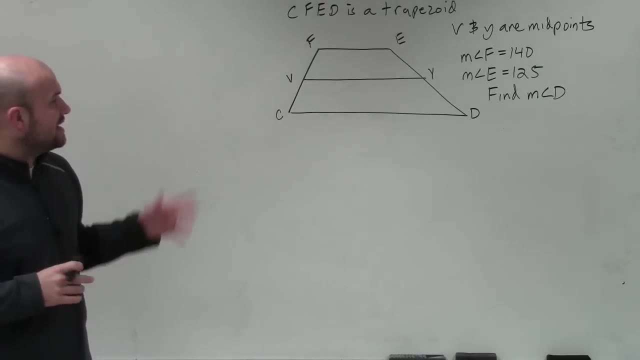 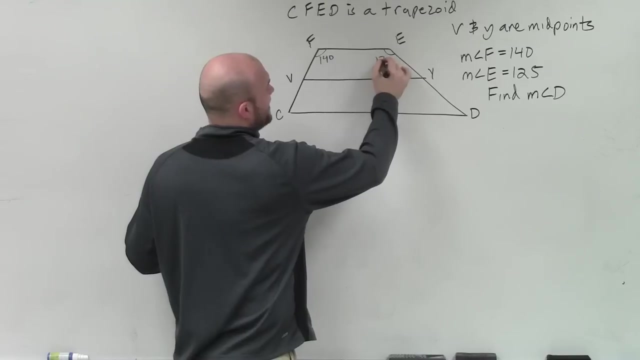 So, on this example problem, ladies and gentlemen, what we have is it says that C, F, E, D is a trapezoid, alright, and V and Y are midpoints. So they say measure of angle F is 140 degrees, measure of angle E is 125, and find the measure of angle D right here. 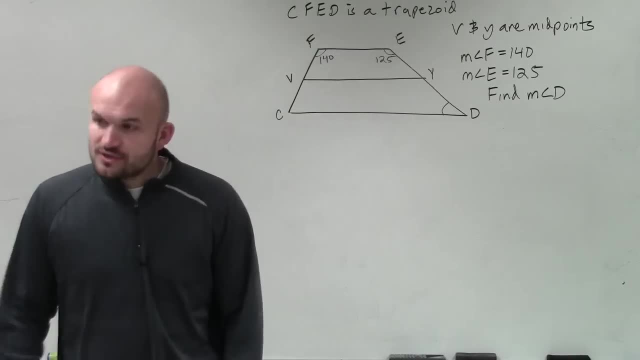 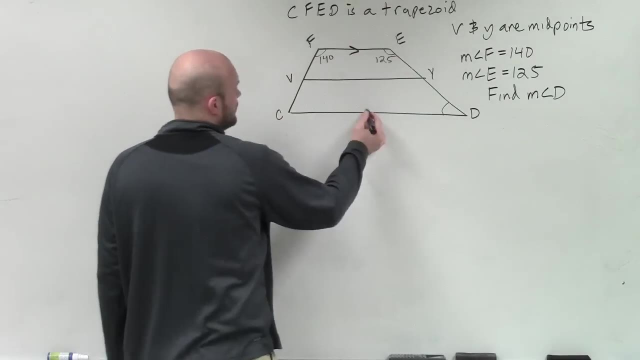 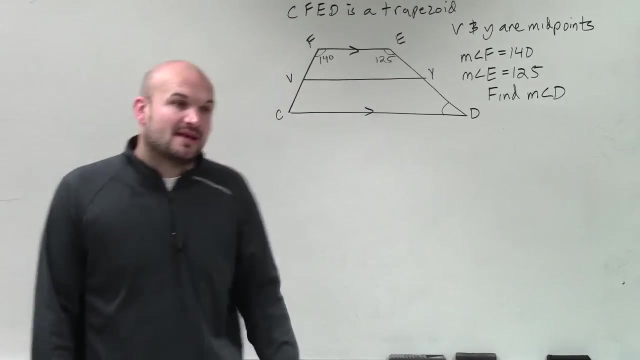 Okay. So there's a couple things that we need to note about this One: it's a trapezoid. Remember trapezoid. we have our bases are going to be parallel right Now. also, remember that, using the mid-segment theorem, that if we have another line that's on the midpoints, that line has to be parallel as well, Correct? 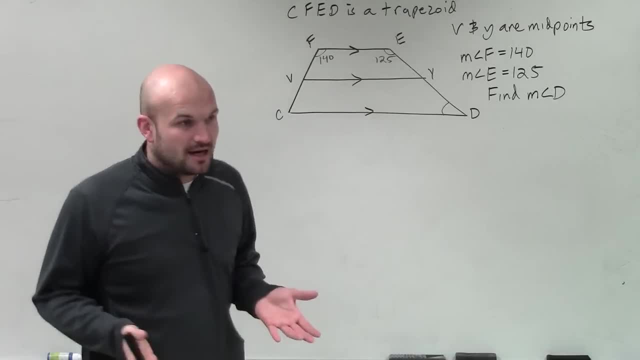 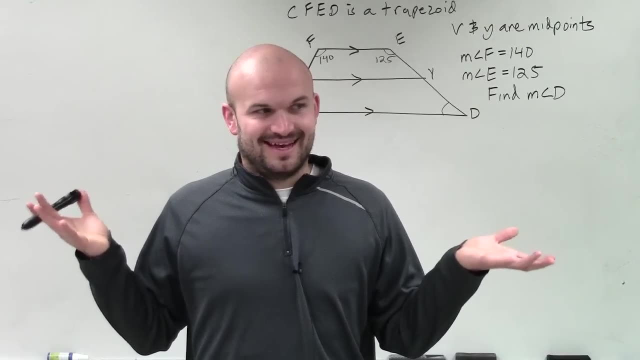 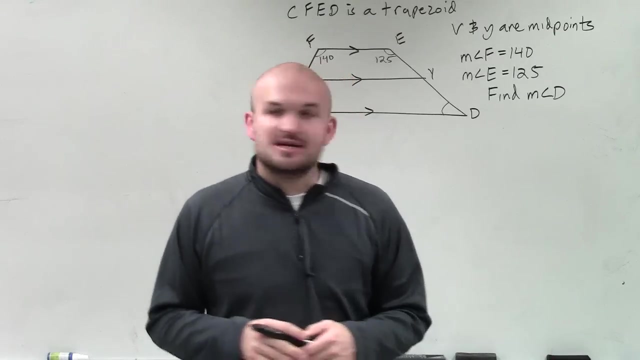 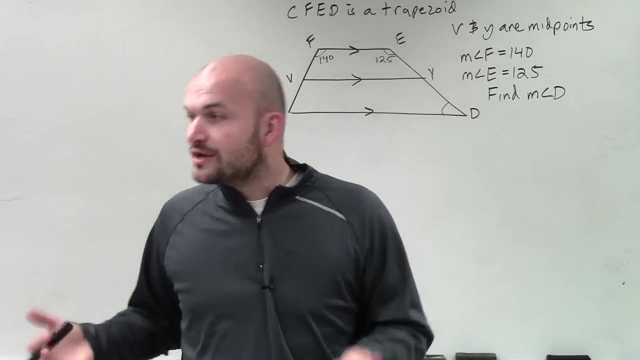 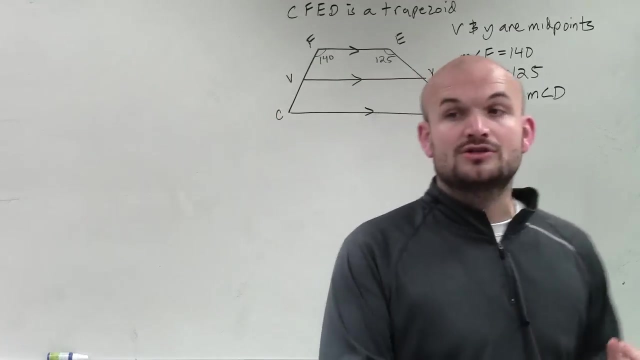 Okay, So by using our idea of parallel lines, remember when we have parallel lines and a trapezoid, If we have a transversal, what is created? Angle relationships, right? One thing I told you guys when we did unit two, with angle relationships or parallel lines, I said: whenever you guys see parallel lines and a transversal, you know there is a relationship. Remember the relationships: alternate interior angles, corresponding angles, consecutive interior angles, alternate exterior angles, right, Those are all created with parallel lines and a transversal. 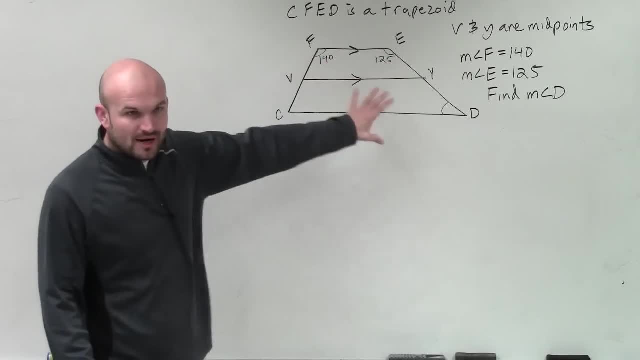 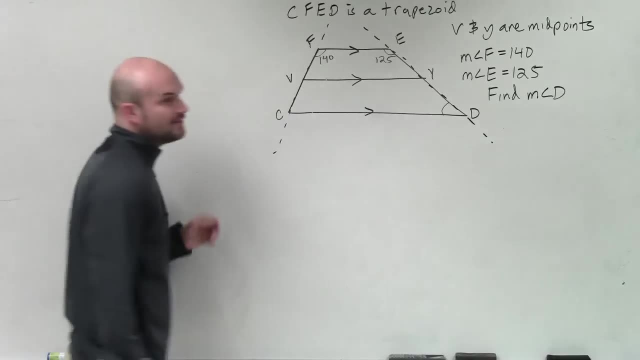 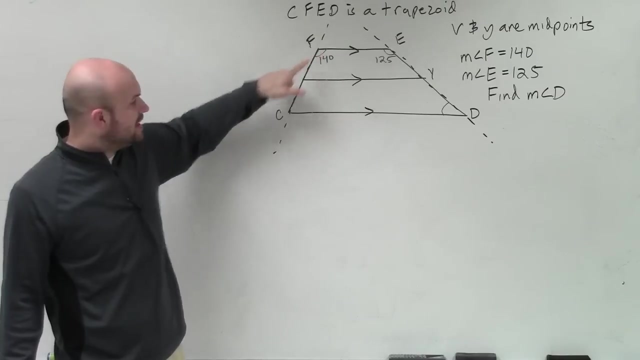 So I know that these lines are parallel and I also have a couple lines that cross them, which we call transversals, right? So if you see, right here here's a parallel lines and then here's a transversal, So if this is 140, what else I could also say that this is 140. And, Zach, do you know why I can say that's 140?? Do you know that angle relationship? 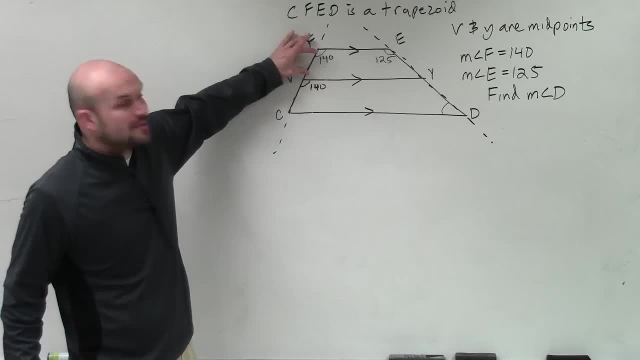 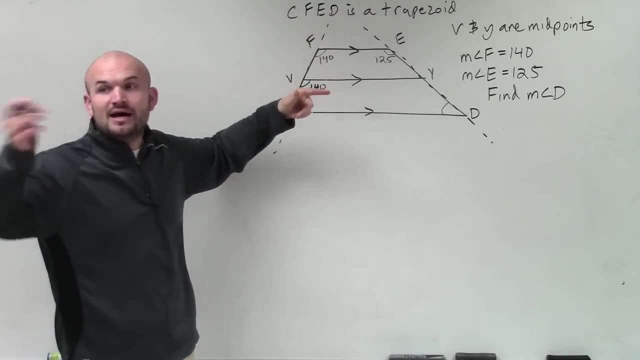 Remember consecutive is consecutive Consecutive interior. So that means both of them would have to be right next to each other, between the parallel lines. So these won't be consecutive interior, but they're in the same spot, in the same parallel lines. Yes, AJ. 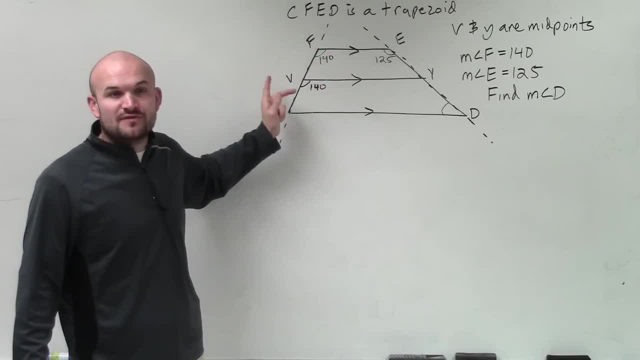 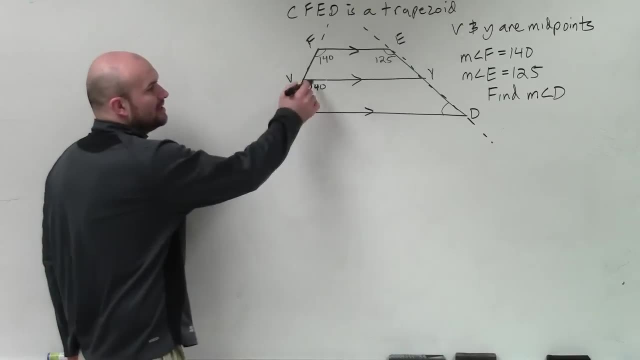 Well, alternate. remember they have to be alternating on different sides of the transversal. So they're still on the same side of the transversal. they're just not both interior Taylor Corresponding right. Very good, So these are corresponding. Then I can also say that over here that's 125, because those are corresponding as well.